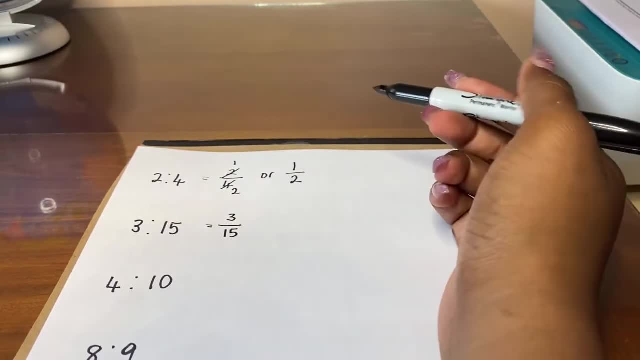 colon. Then we're going to look at these two numbers and figure out what is the highest common factor that can reduce it. So the highest number that can go into both 3 and 15 is 3.. So we're going to say: how many times can 3 go into 3?? 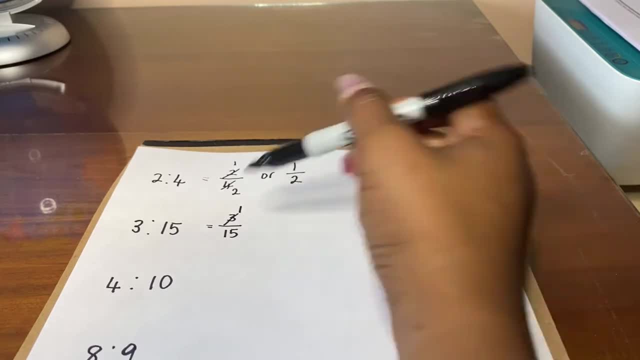 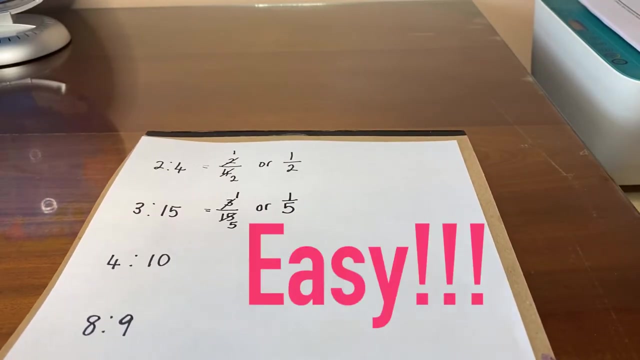 One time. How many times can 3 go into 15?? That's 5 times. So 3 to 15 written as a fraction is 1 over 5.. All right, Moving on to the third ratio. Pretty easy, huh. We have 4 to 10.. 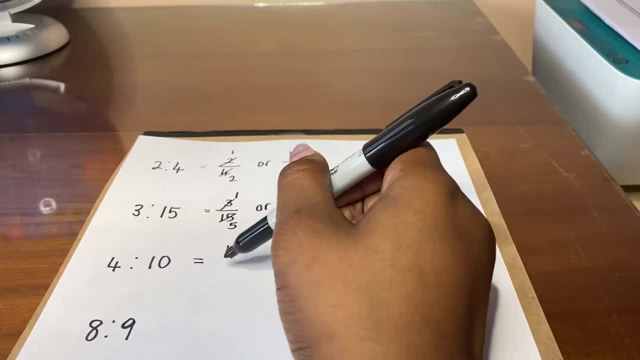 Again, we put the first term as the numerator and the second term as the denominator. Then we're going to look to see how many times can 3 go into 15.. So 3 to 15 is 1 over 5.. 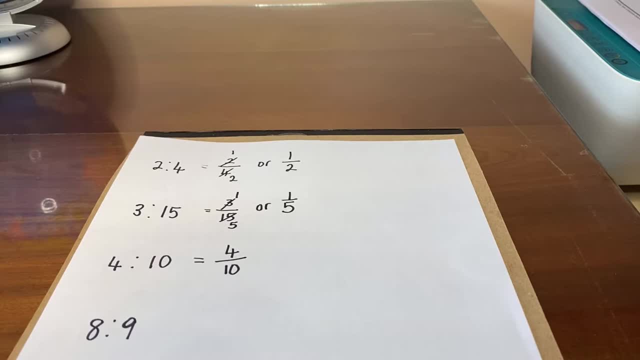 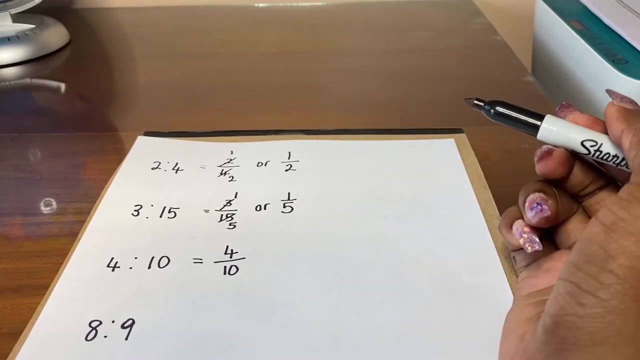 And then we're going to see if this fraction can be reduced to a lower term. And yes, So the highest number or the greatest factor that can divide both 4 and 10 is, if you've guessed, 2, you're correct. So we're going to say: how many times can 2 go into 4?? 2 can go into 4 two times. 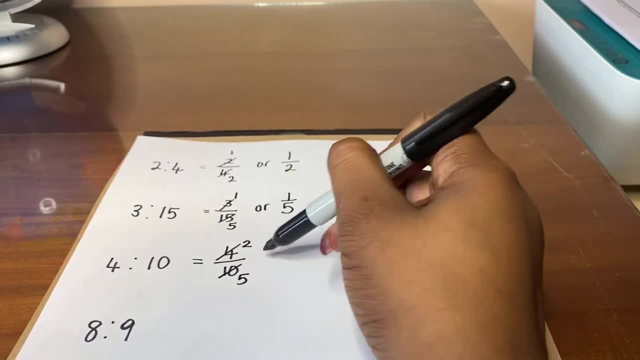 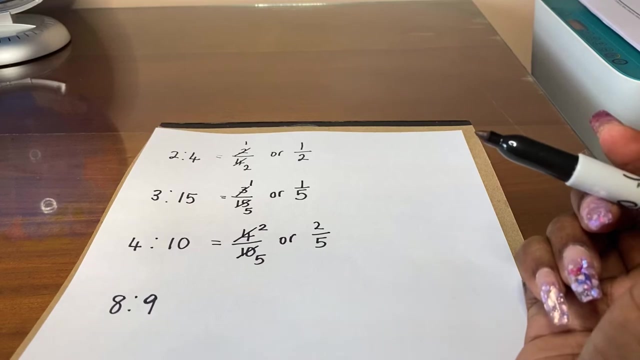 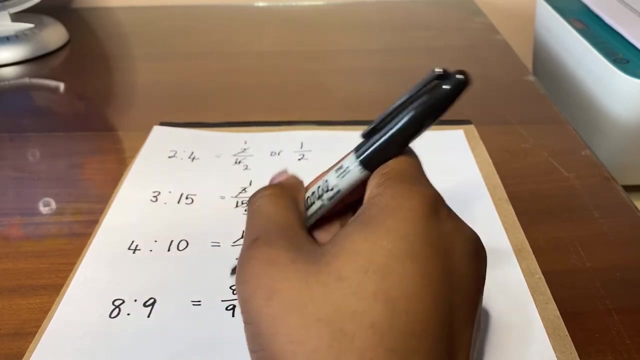 and 2 can go into 10 five times. So 4 to 10 as a fraction is 2 over 5.. All right, Then we're going to look at our last ratio that we'll be looking at for this video. So again, we're going to put 8 over 9, because the first number is the top number. 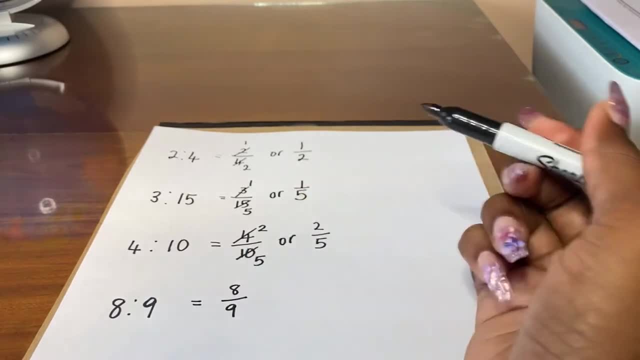 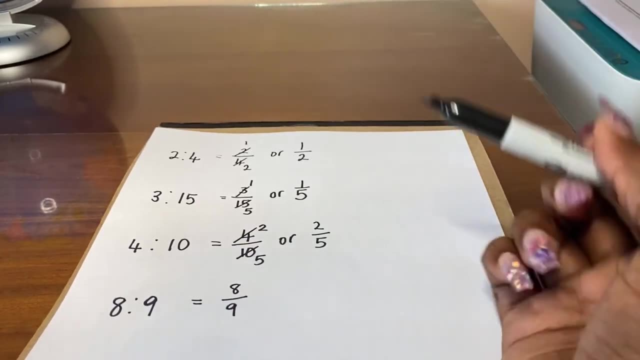 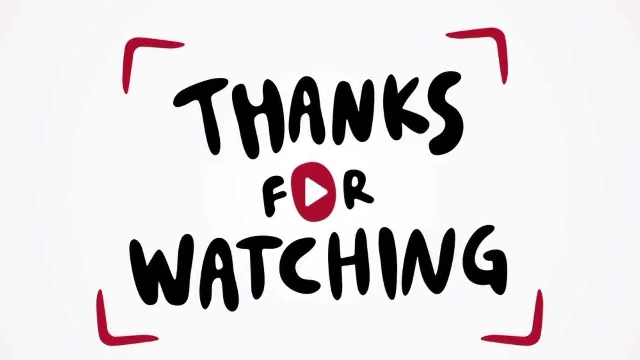 the second would be the bottom, And then, looking at this, there's not a number that can divide both 8 and 9 without leaving a remainder. So therefore, this fraction stays, as is All right. Thank you so much. If you found this video very helpful, go ahead and give us a thumbs. 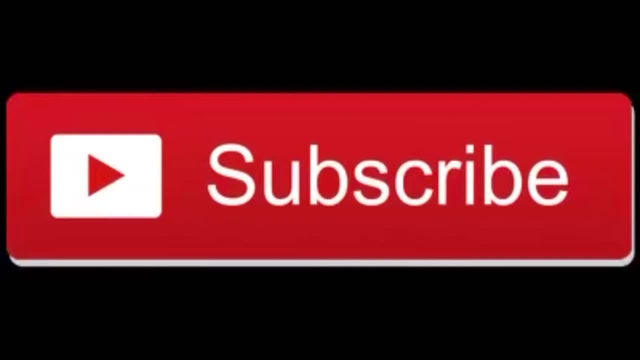 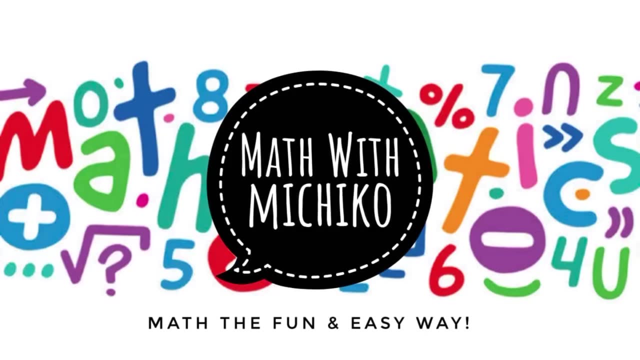 up. Ensure that you subscribe for more fun and easy math content coming your way. Be sure to comment down below and let us know the topics that you'd like us to explore. Thank you and bye.